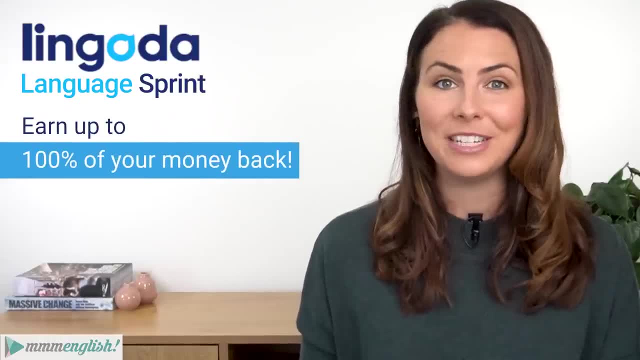 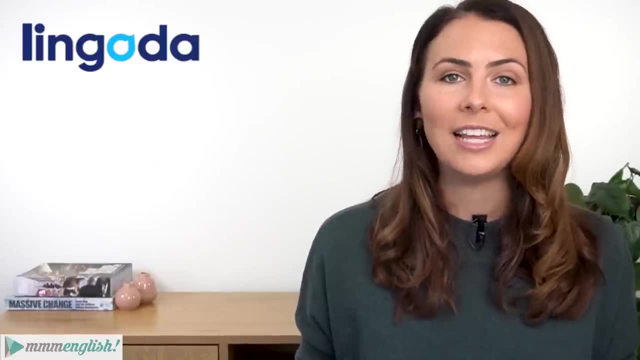 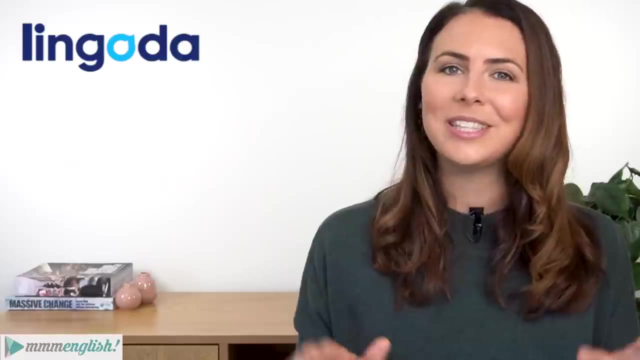 and find out how you can get a 100% refund on your class fees by checking out this video up here. Of all the places that you can learn a language online, Lingoda are, in my opinion, one of the best. Anyone who watches my channel regularly knows that I've taken plenty of Spanish. 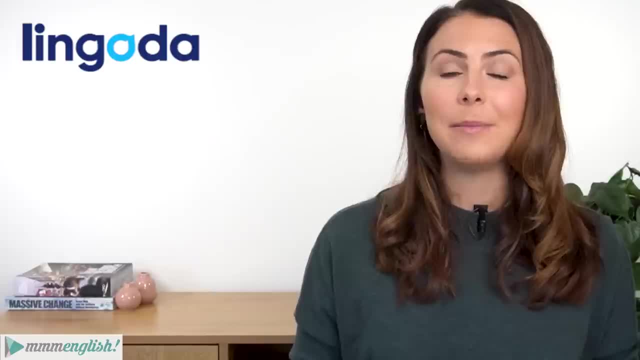 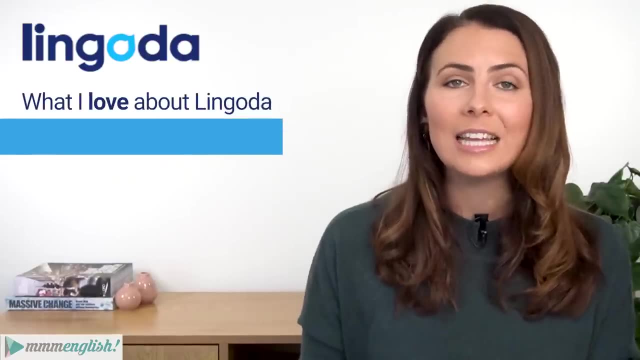 classes with Lingoda myself, and I've also spent some time exploring the English curriculum and teaching methods As a teacher. what I love about Lingoda is the clear structure of their lessons. You always know what you need to do next and you're always working your way. 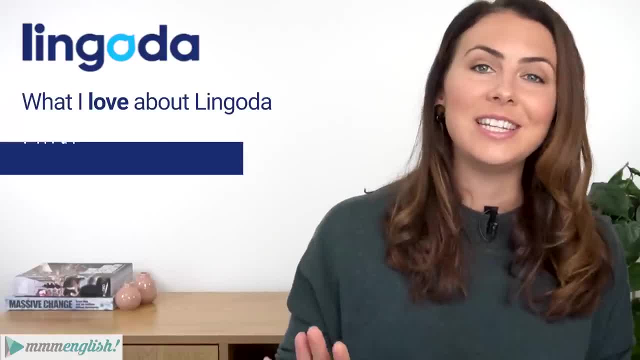 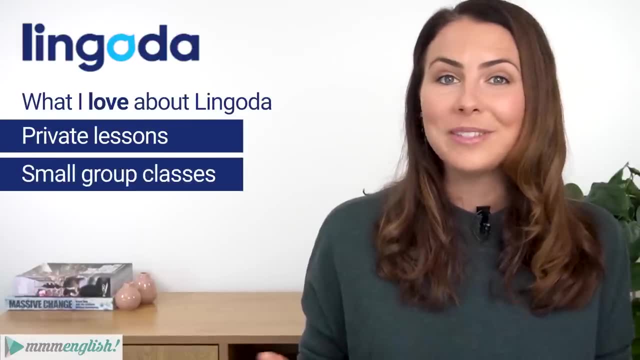 towards your next certification. If you're interested in private one-to-one lessons, you can take those with Lingoda, but if you prefer to learn in small groups and meet other people well, you can take group classes as well. All of Lingoda's classes: 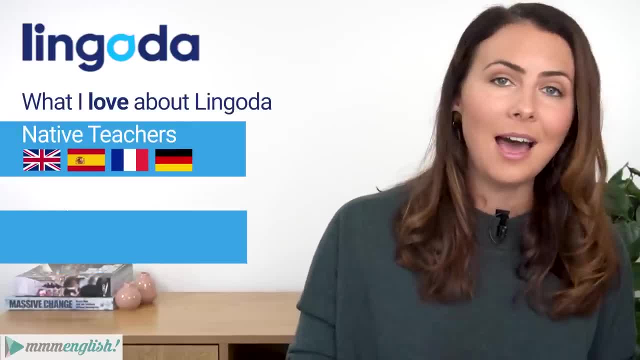 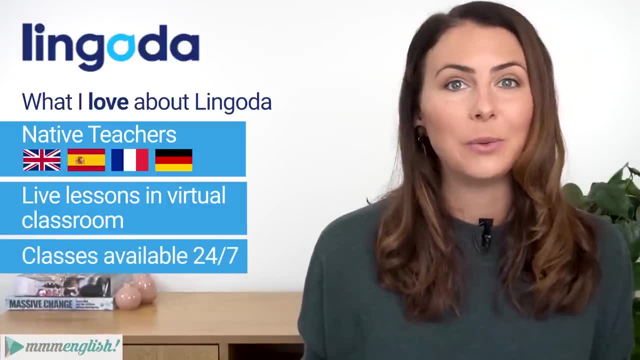 are delivered by native teachers and each one is live. it's interactive, so you can participate, and there are classes available 24 hours a day, seven days a week. So if you'd like to try it out, there are a couple of ways that you can get started. 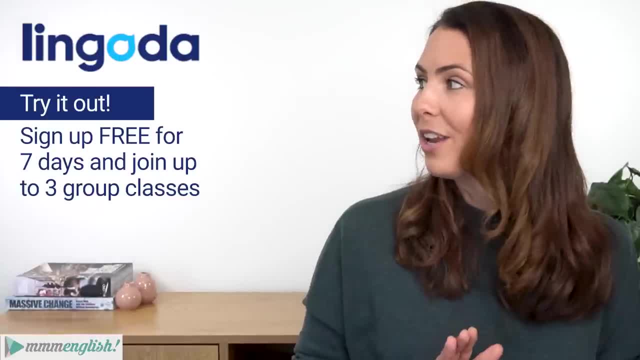 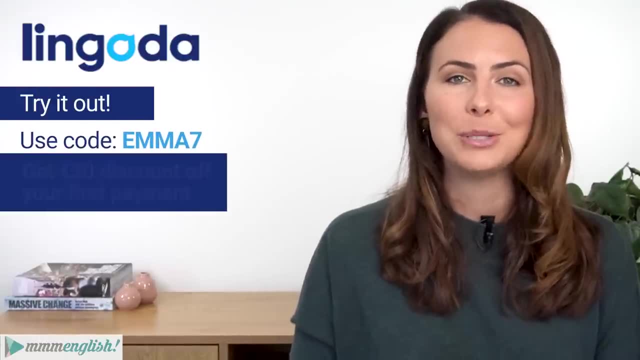 You can sign up for free for seven days and join up to three group classes, or you can use this code to get a 20 euro discount off your first payment. I'll put all of the links into the description below, but it's definitely worth checking out. 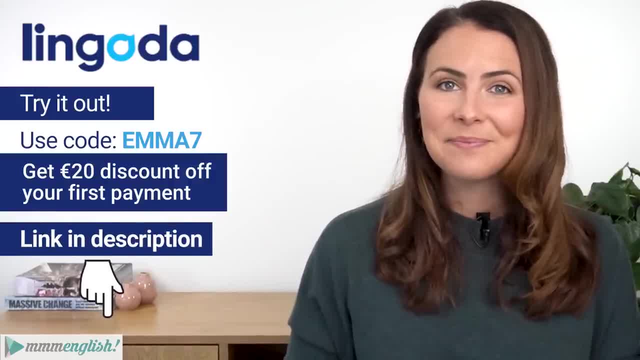 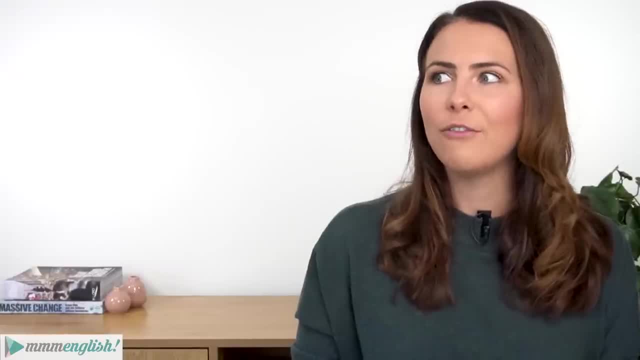 It's definitely worth taking a look. Let me know what you think. All right, it's about time we got started and we're going to go through some collocations and some common expressions for when we have time, when we have enough or we have lots of time. So, of course, 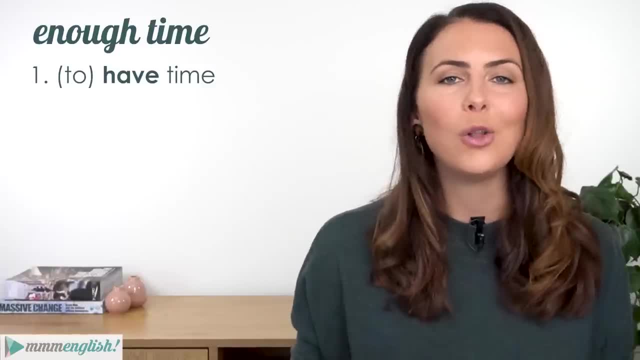 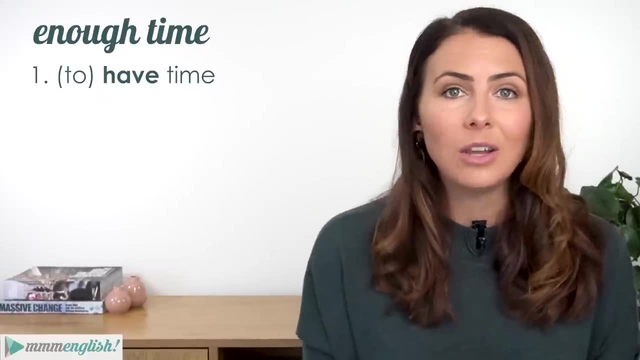 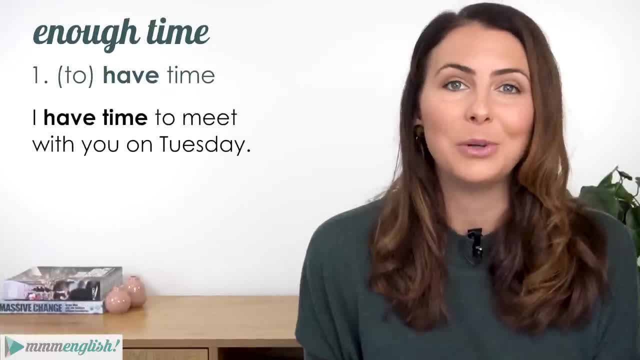 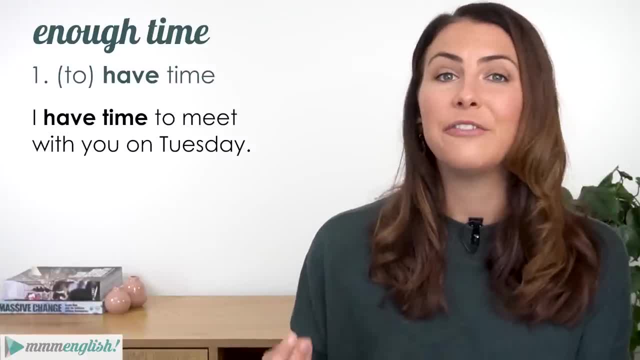 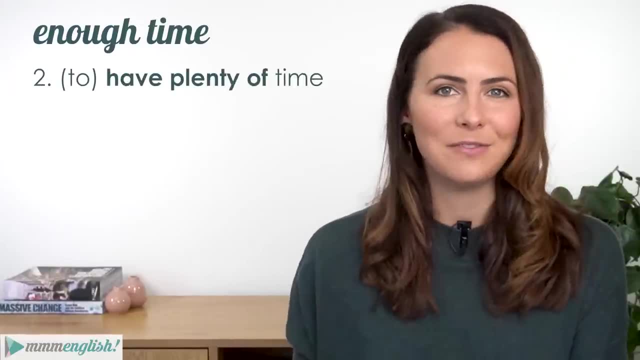 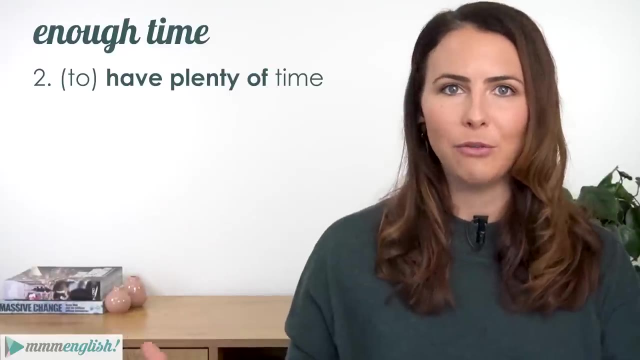 expressions that use have time, these fixed expressions. So when you've got more time than you need, you have plenty of time, plenty of time. Not only do you have time for something, but you've got a lot of time available for it. 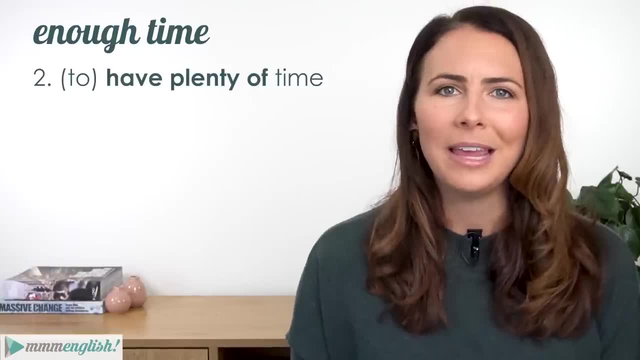 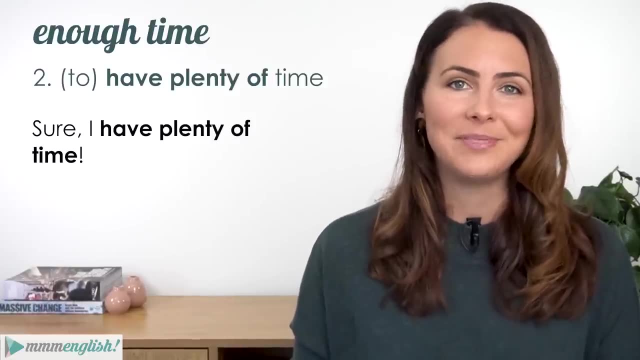 So if someone said to you, are you sure you don't mind helping me, You could say: sure, I have plenty of time, or I've got plenty of time, I can help. Another way to express the same thing is to say that you have. 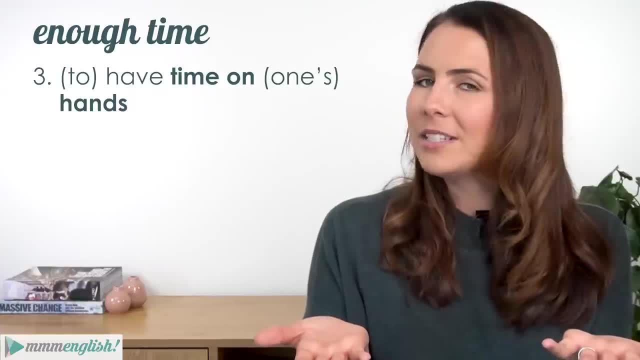 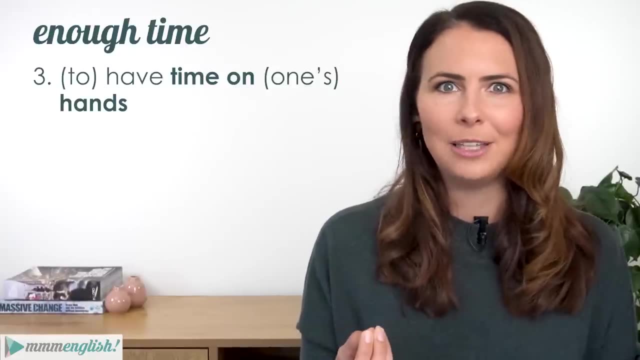 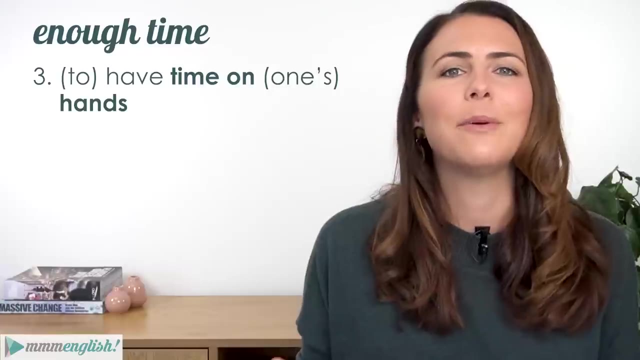 time on your hands. Now, this is a pretty casual phrase. It's often used when you find yourself with some unexpected time available. I had some extra time on my hands, so I offered to manage the community garden. And if you want to be really dramatic and exaggerate how much spare time you have, 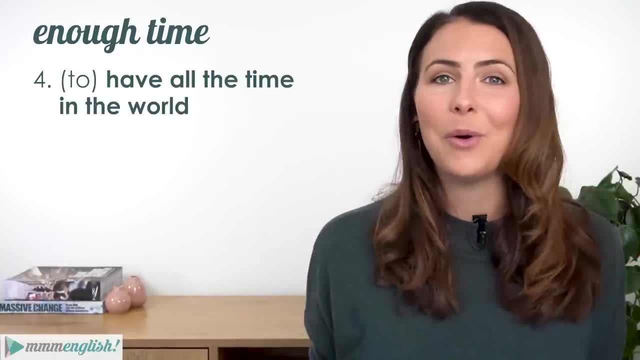 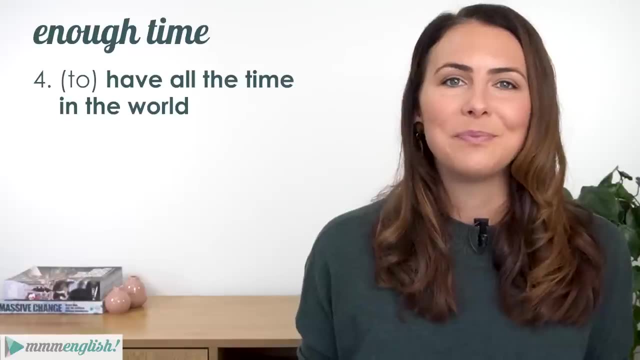 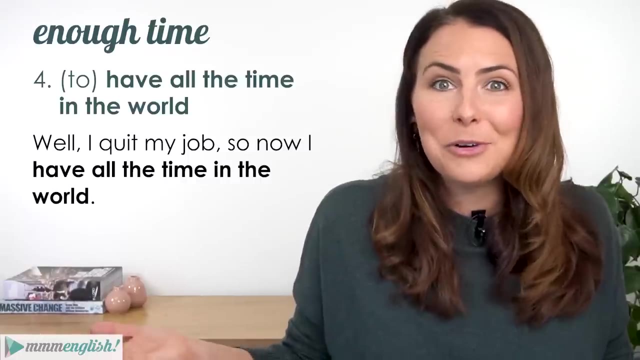 then you could say that you have all the time in the world. Now, this expression is often used sarcastically, you know, to make a joke. So if I said: what day are you free to meet this week? Well, I quit my job, so now I have all the time in the. 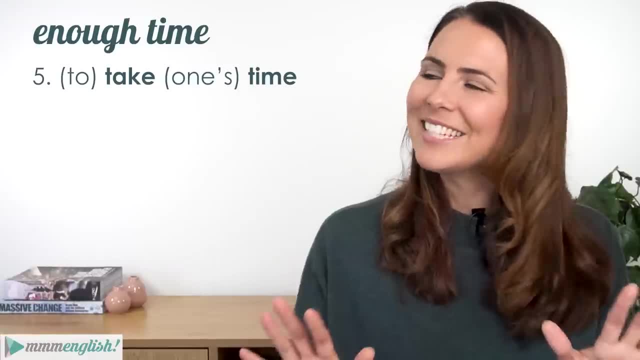 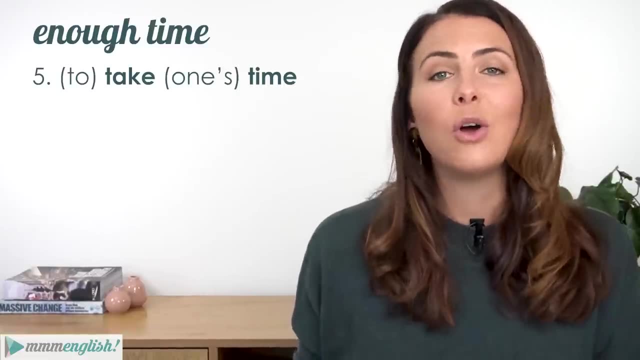 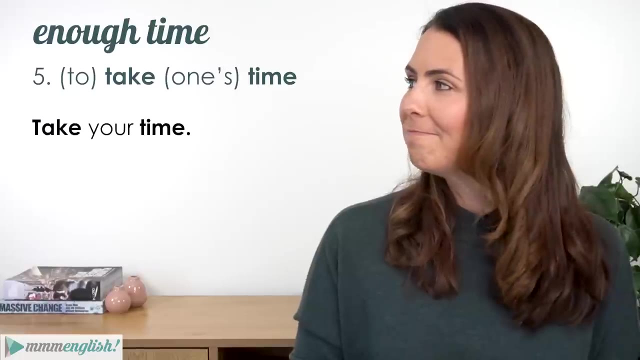 world: Take your time Now. this expression is useful when you want to tell someone else to relax. You know they don't need to stress because you're not worried about how long it may take. You have the time to wait. So you say: take your time- Another way to use this. 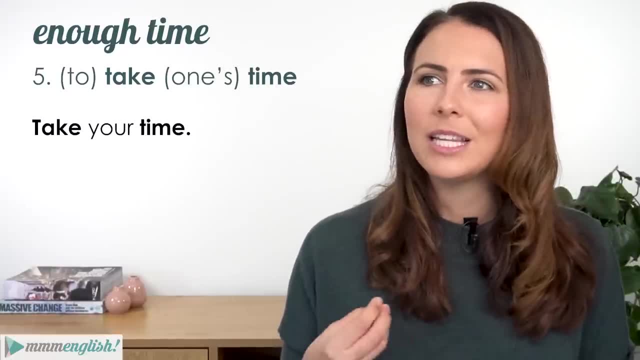 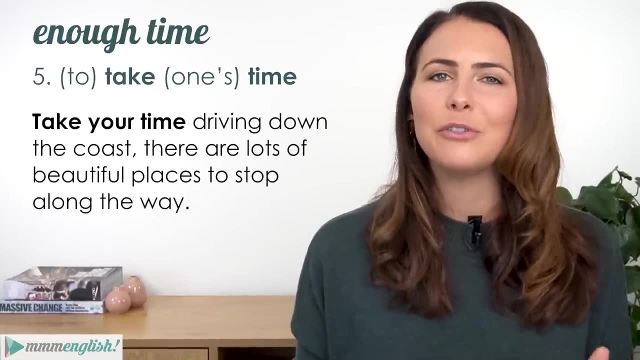 same expression is when you're doing something really slowly because you're really enjoying it. Take your time driving down the coast. There are lots of beautiful places to stop along the way. Oh, and pay close attention to that verb If you choose to use. 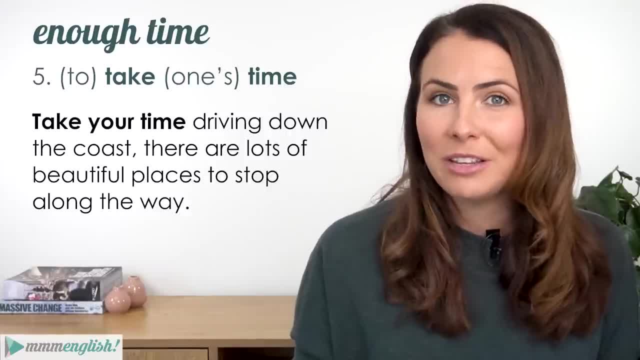 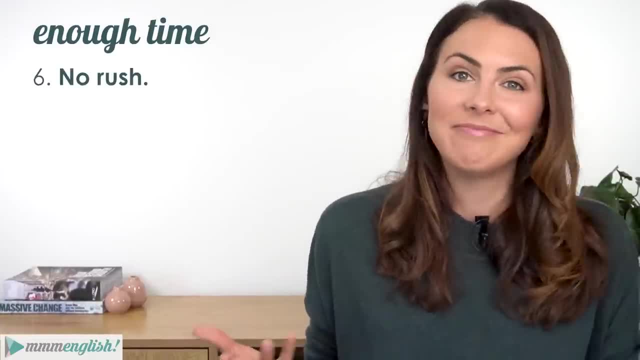 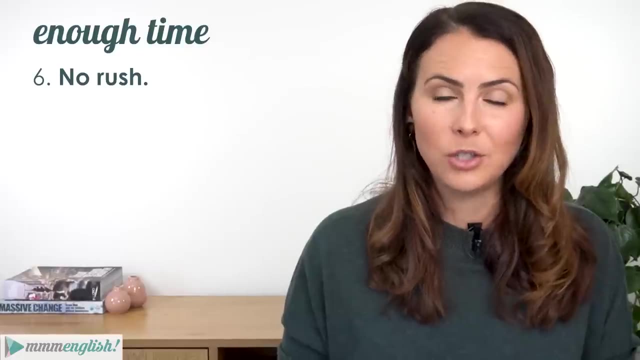 a verb with this expression, then you need to use the img form, not the infinitive No rush. This is another informal way of saying kind of the same thing. to take your time, No rush, There's no rush. This is a fixed expression, so it's always used in this way. 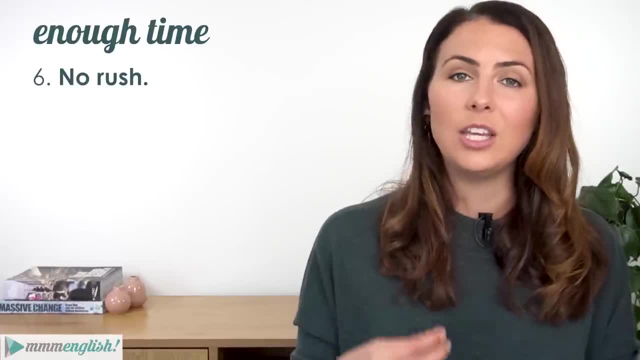 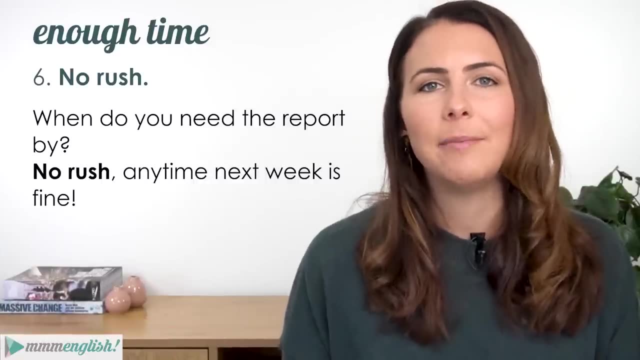 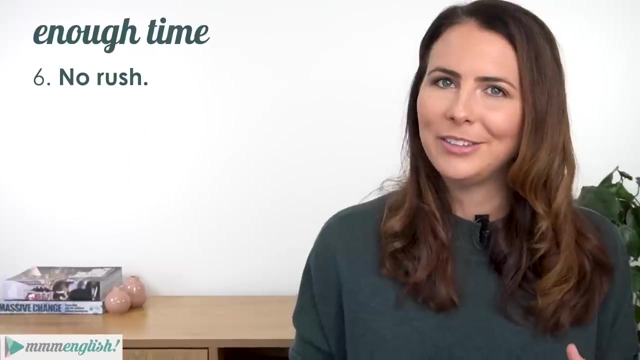 kind of casually, and it's usually something that you tell the other person. When do you need the report? by No rush. Next week is fine. Now, when you're talking about yourself and your own actions, you need to include a preposition. You 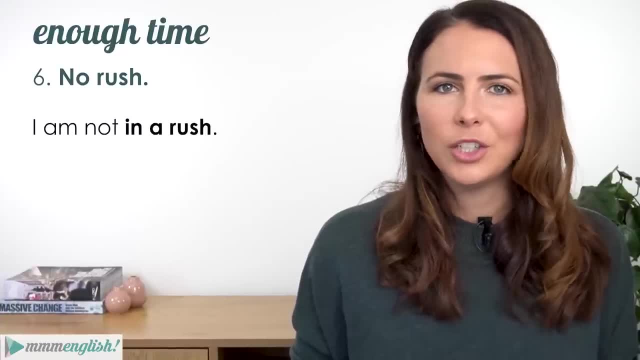 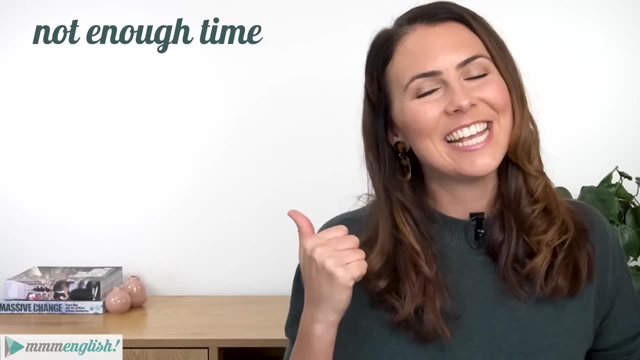 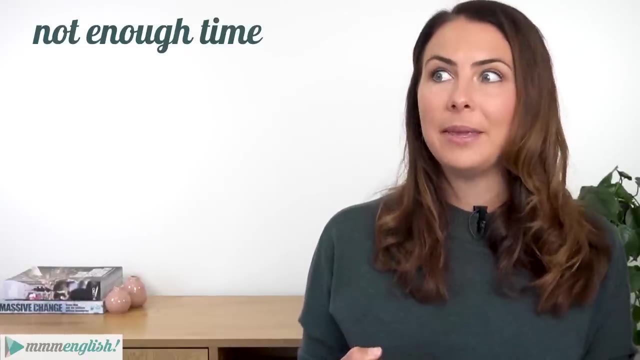 need to say I'm not in a rush. I'm not in a rush, No rush, I'm not in a rush. Okay, on to the second list. now I told you we'd be moving quickly, So we just talked about having time, maybe having lots of time, but now we're. 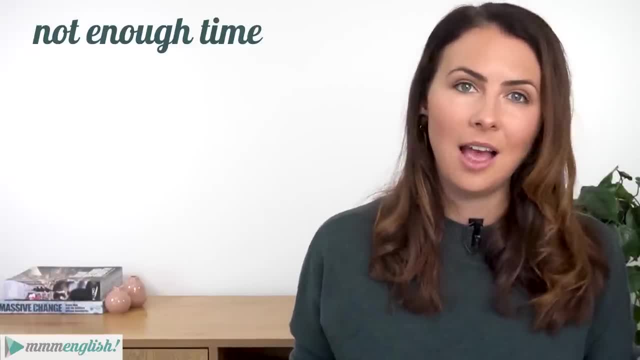 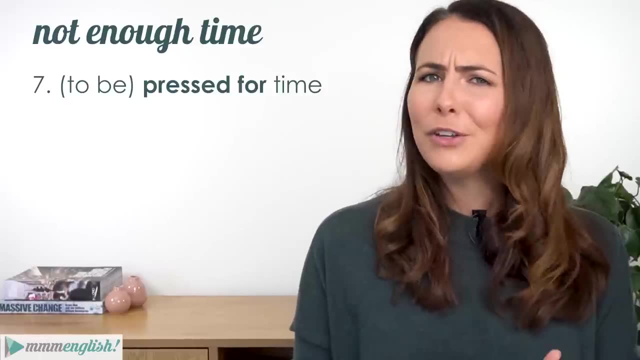 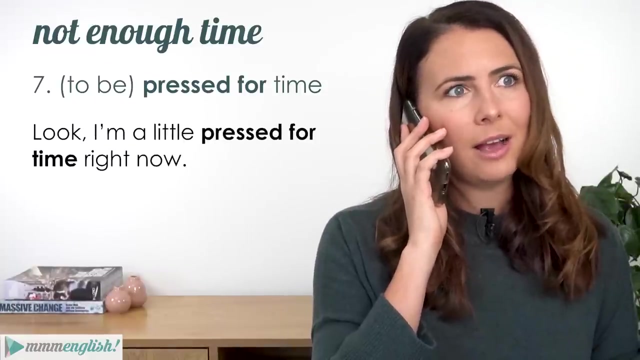 going to talk about the opposite. when there's a lack of time, We don't have enough time, So in those situations you can say that you are pressed for time. It's often used as a way to remind someone to hurry up, to go a little bit faster. Look, I'm a little pressed for time right now. 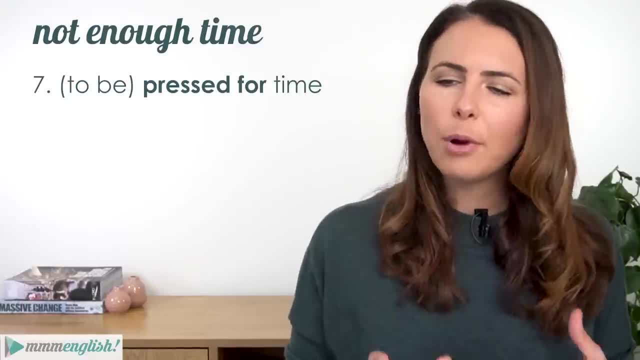 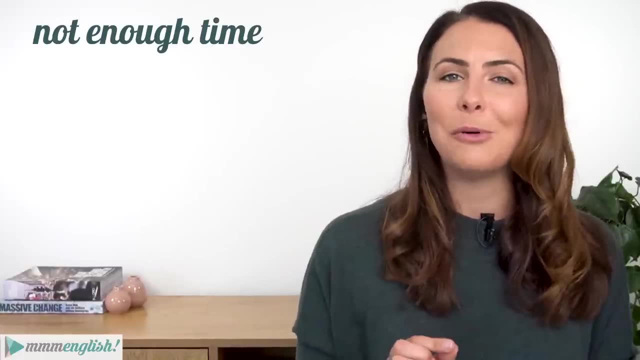 Can you just give me a call back once you know the answer? So it's probably a little formal. so it's great to use in a professional context at work. If you want something more informal, then you can say that you are short on time. 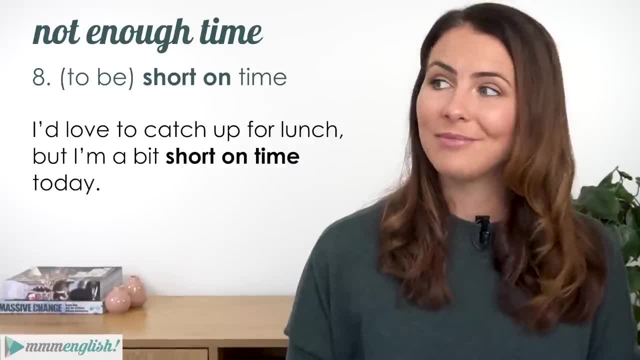 I'd love to hear your thoughts in the comments below. I'd love to hear your thoughts in the comments below. I'd love to catch up for lunch, but I'm a bit short on time today. Can we meet next week instead? Oh, when you're running out of time, you're going as fast as you can. 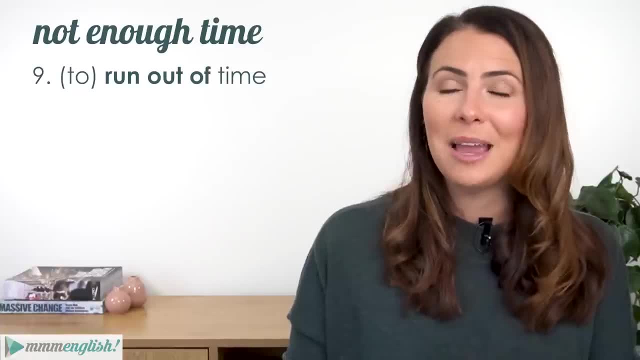 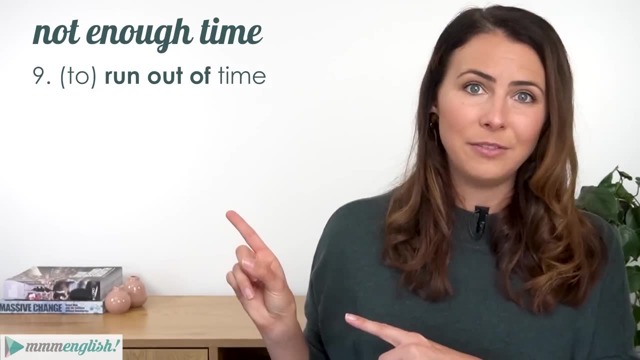 but you have to finish something. You don't have enough time to do it. The time that you need to do it by is getting closer and closer and closer, so you're running out of time. Now you use the continuous version when there's still a little bit of time left. 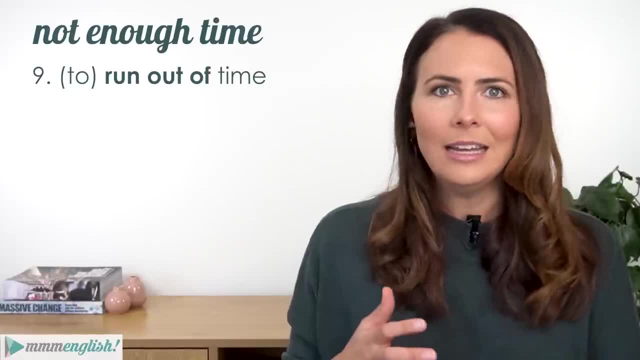 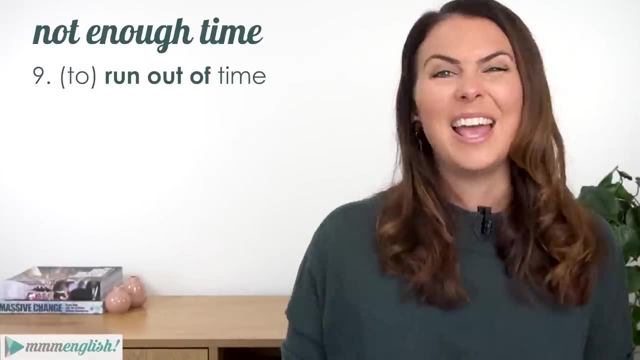 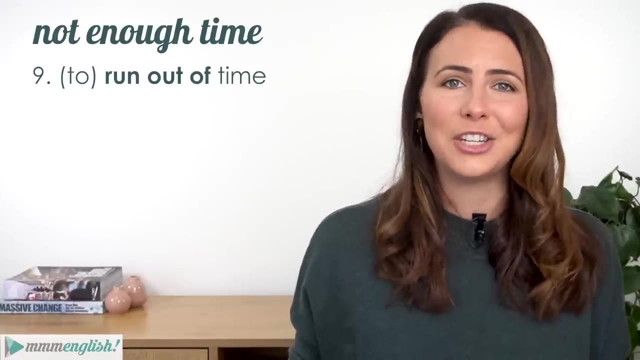 but it doesn't seem like enough. You know it's like hurry, we're running out of time. We've still got a little bit of time, but there's not much time left and we use the past tense when that time is already over. you know We can't finish the action now. it's too. 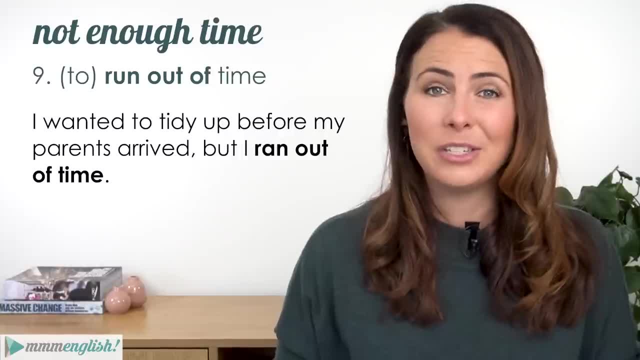 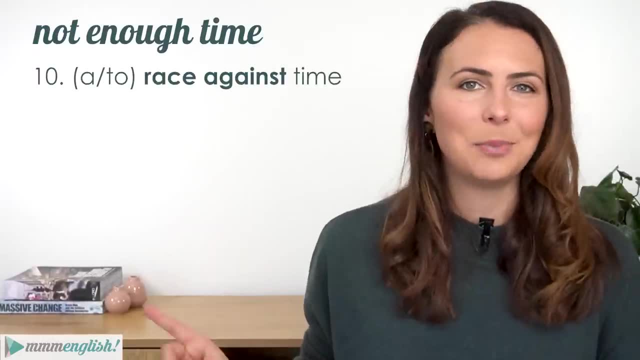 late. I wanted to tidy up before my parents arrived, but I ran out of time so I never actually got to complete the action. This is another great expression in this situation: When you're panicked, you're trying to finish before you run out of time. 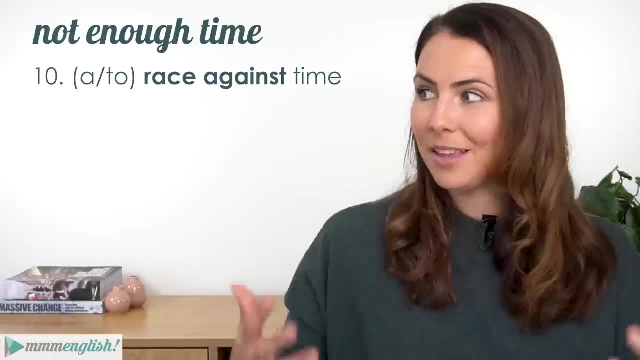 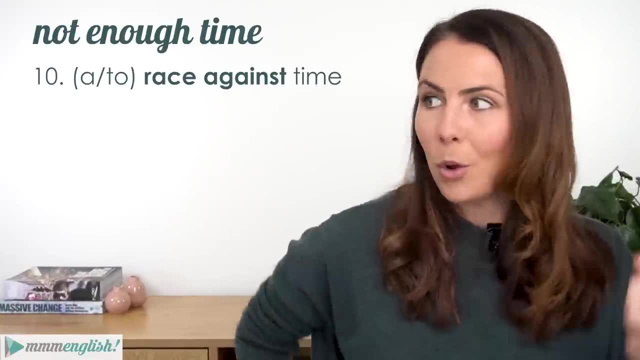 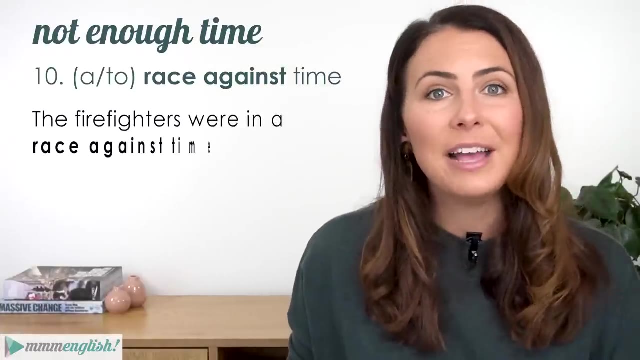 well then, you're in a race against time, Me versus time, right? Imagine that you are in a race with time. Who's going to win that race? You know a literal race: You or time. The fire was moving quickly towards the town, so the firefighters were in a race against time. 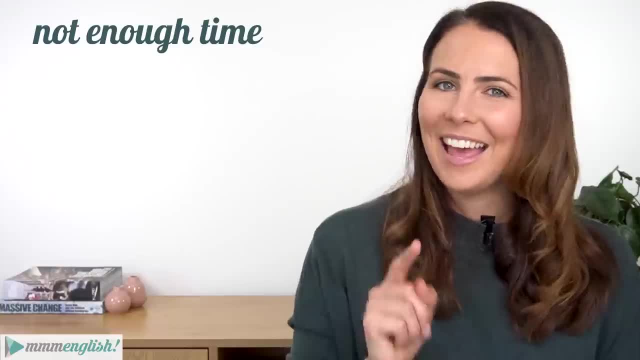 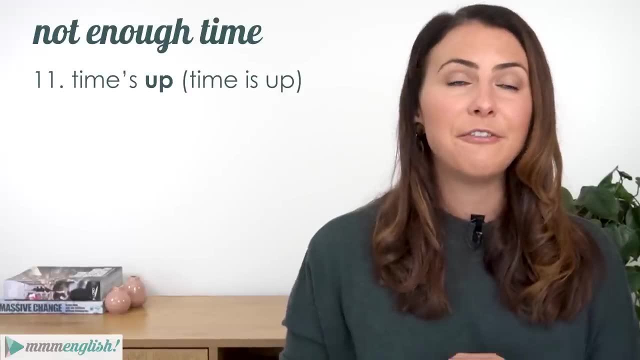 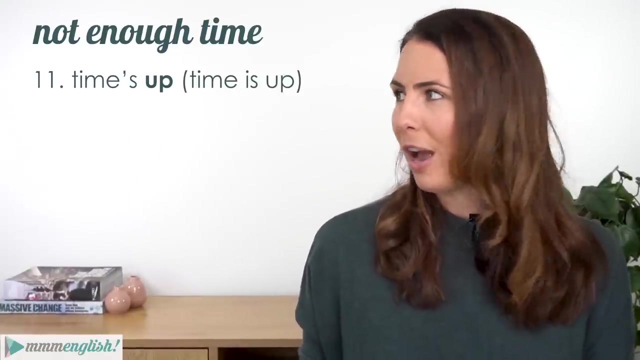 or they were racing against time. And if you do run out of time, then time's up. Time's up is what we say when there is officially no more time. You can't continue Now. it's almost always said in the contracted form. 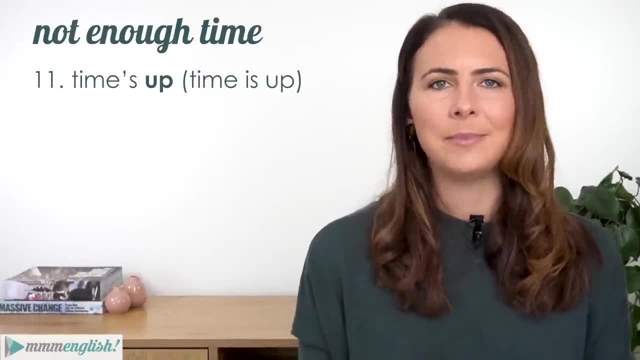 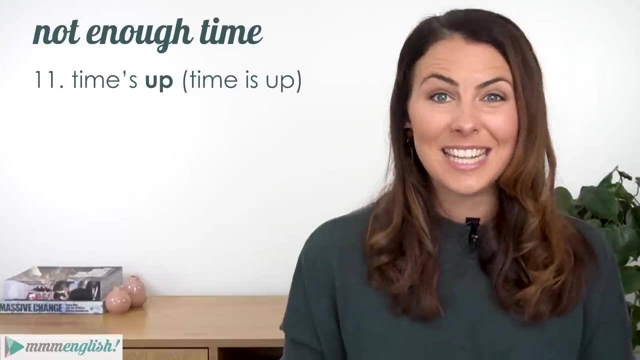 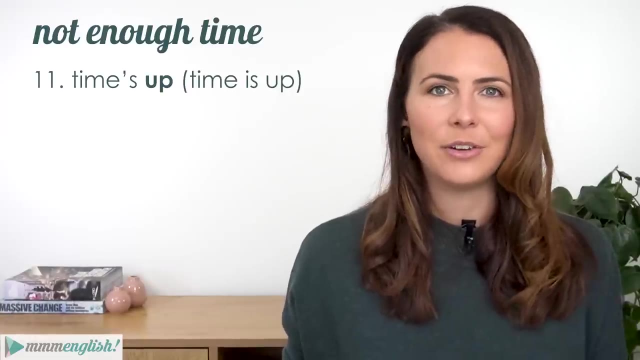 Time's up. Not time is up, but time's up, And it can be used as a way of saying stop, like when you're playing a game or when you're sitting an exam and the time finishes. If it was a one-hour exam, the exam finishes after an hour. put down your pen. 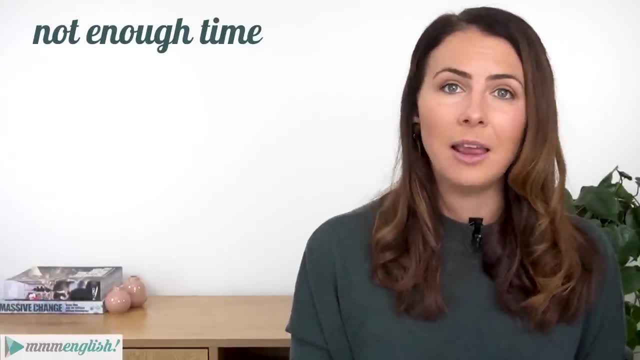 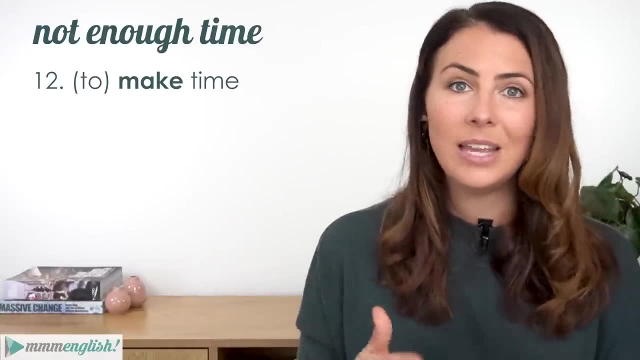 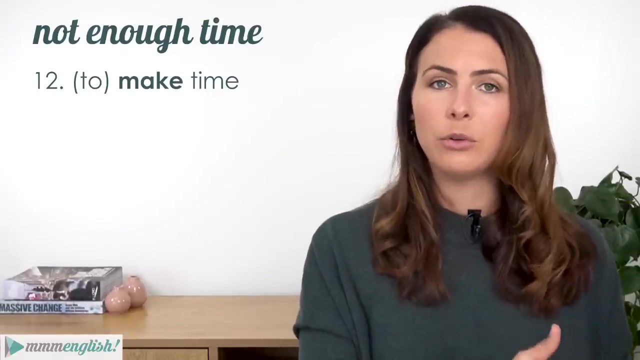 time's up Now if you don't have time, but it's really important that you create some time. you need to make time Now. it suggests that you need to make a decision not to do something in order to create that time or to create the opportunity to do something. 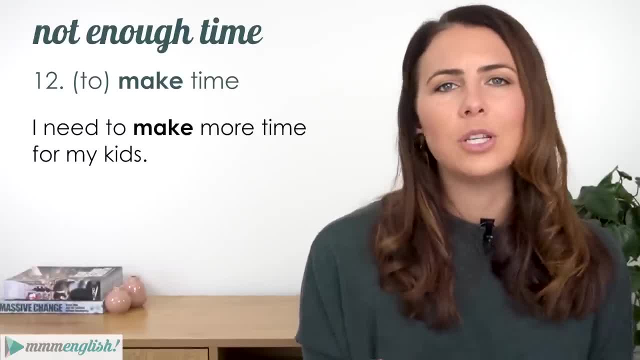 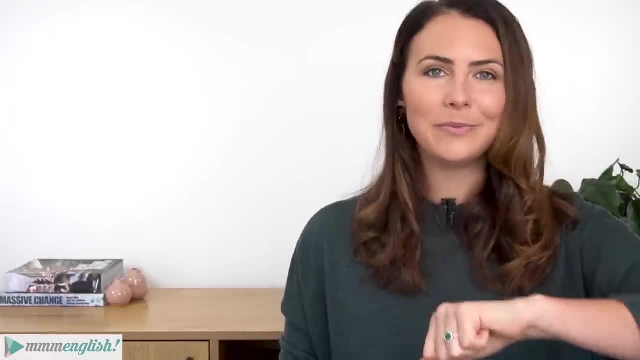 So you'll often hear people saying: I need to make more time for my kids. I know it's really important for you, so I'll make time to do it. Whoa, Time is flying, And that is our next category: time passing quickly. 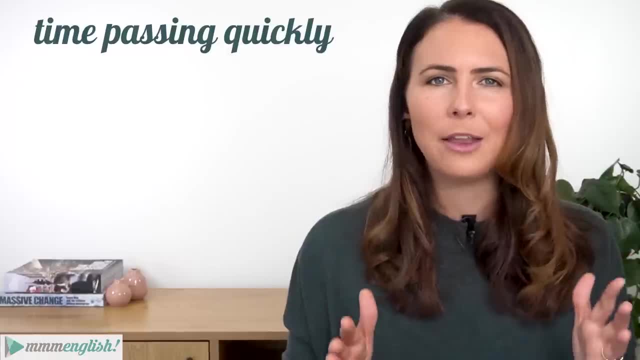 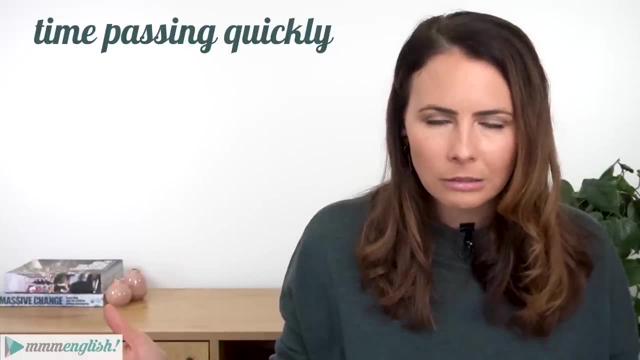 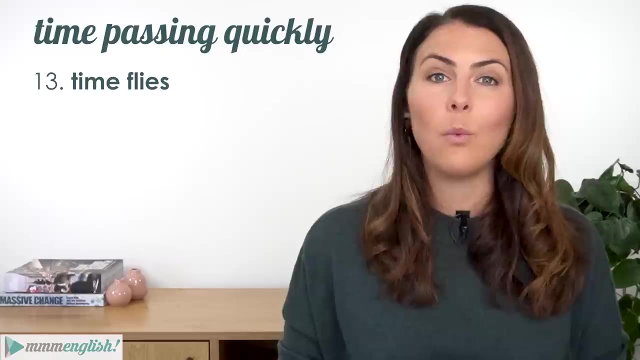 Don't you think that it's really weird that the same actual amount of time can pass really quickly for one person and then really slowly for another? That's what we're going to talk about now. So time flies and we use the continuous tense when whatever we're doing in that moment feels like it's happening really, really quickly. 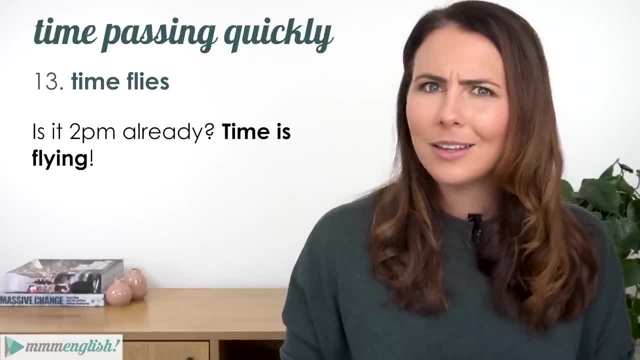 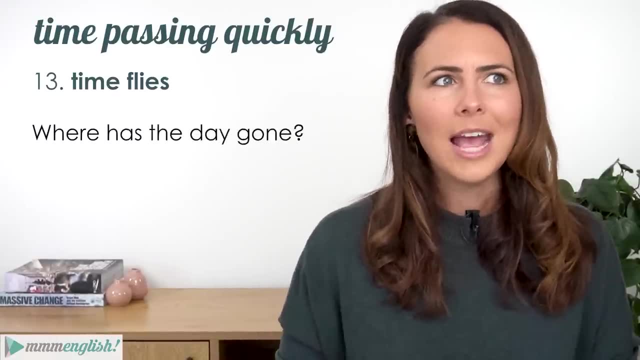 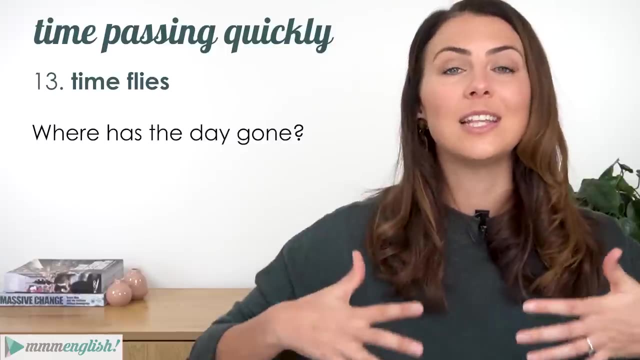 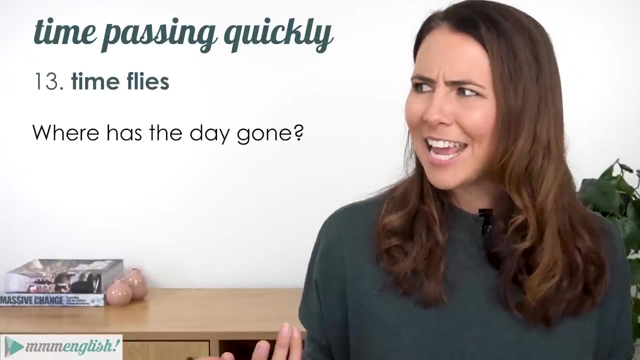 Is it 2 pm already? Time is flying. This is also when you start to hear strange expressions like: Where has the day gone? Like the day's disappeared. but it's just that time is disappearing so quickly that it feels like half the day is gone. Where's the day gone? And we use the simple present. 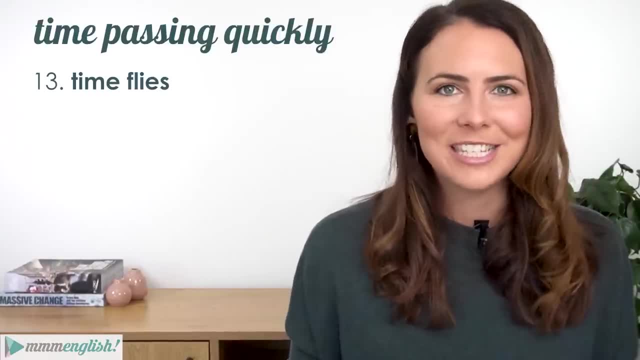 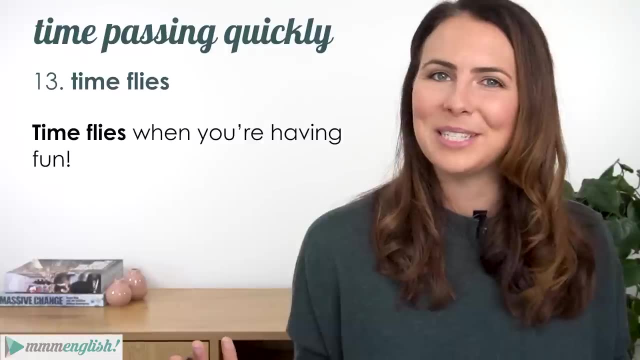 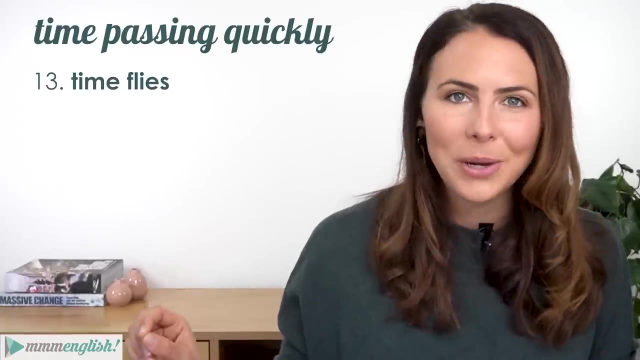 Time flies, to make a general expression statement about when time passes quickly. Time flies when you're having fun is a common expression and it's often shortened to simply time flies, And when time passes so quickly when you're doing something that you're so interested. 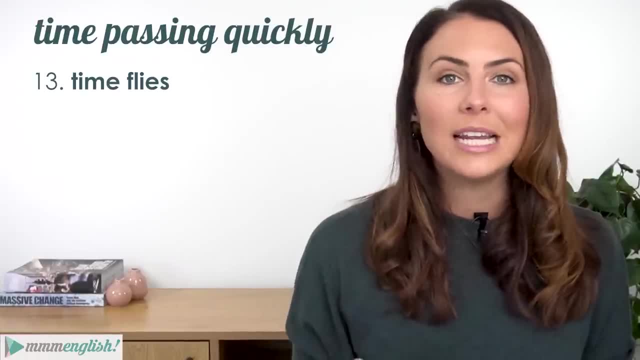 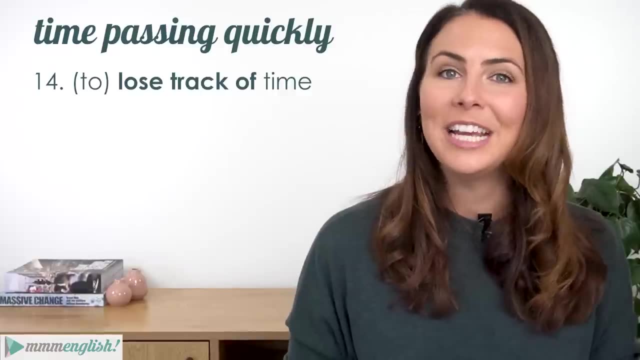 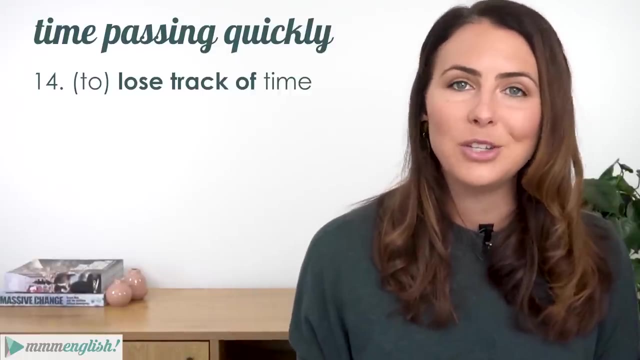 or you're so involved in doing that you don't realise how much time has passed. then you lose track of time. You've heard me talk about this expression before. It's usually used in the past tense, after you finally have taken a break from whatever you've been doing. 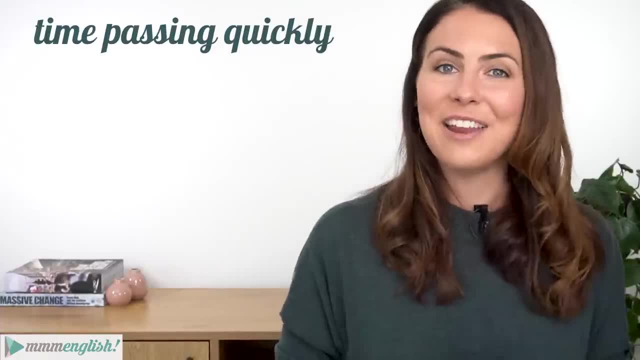 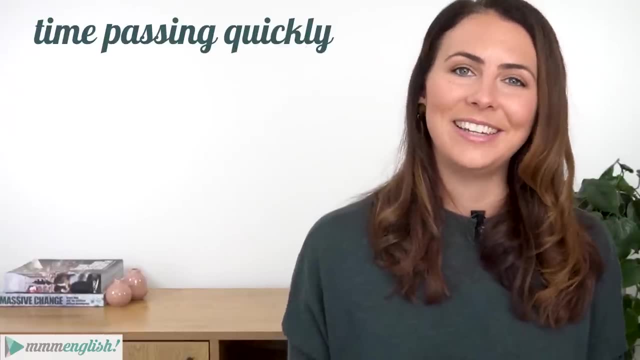 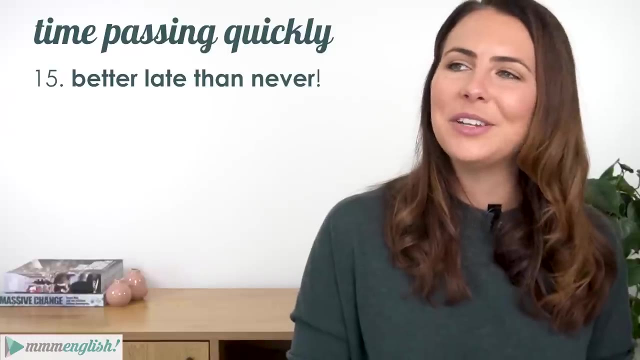 and you suddenly realise how much time has passed. And finally, if you did lose track of time and you complete a task or something after you should have done it, then the best phrase to use is better late than never. So this expression is quite a good, informal or friendly apology. 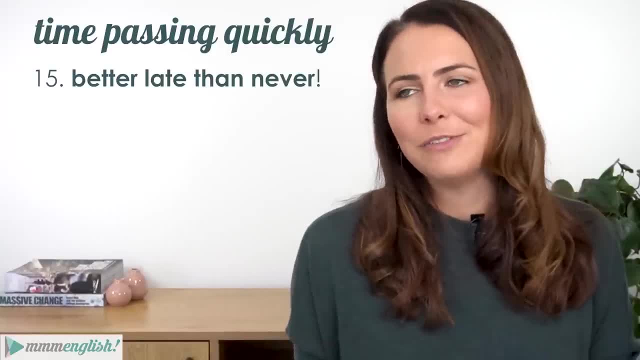 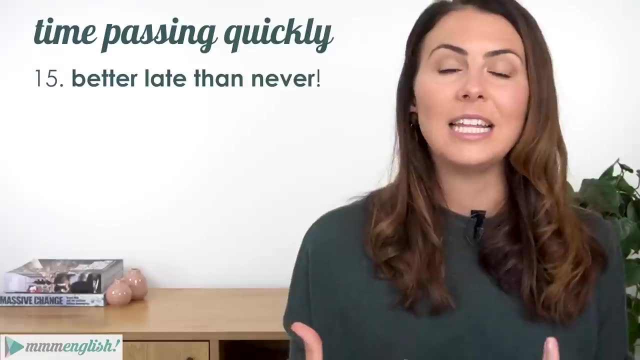 to remind someone not to get upset because you've done something late. The fact is it got done and that's a good thing. So this is a fixed expression that doesn't really need further explanation. So just imagine that your friend's birthday was last month. 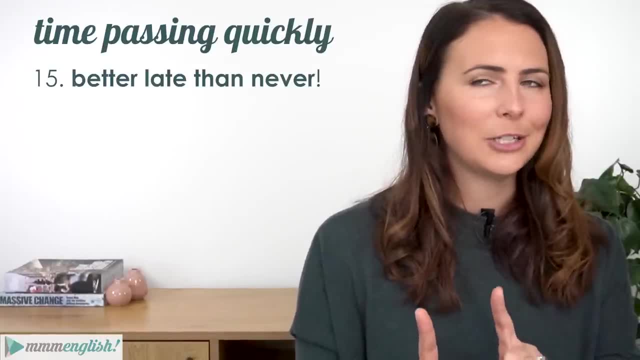 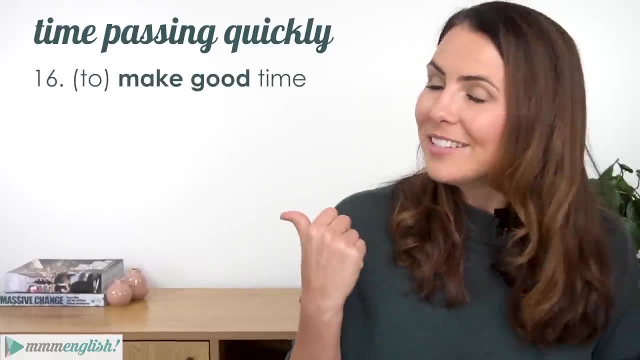 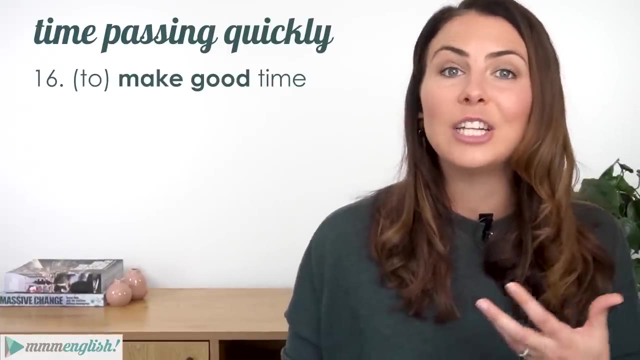 and you completely forgot about it. so you bought an extra special present to make up for it, and you could say: better late than never, right? So this expression is used for trips, you know, when you're on some kind of journey or a trip and you're actually getting there faster. 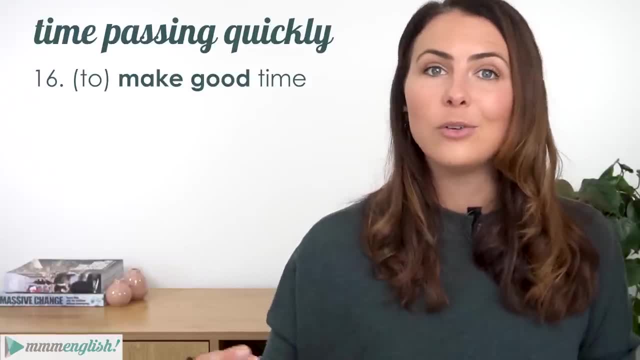 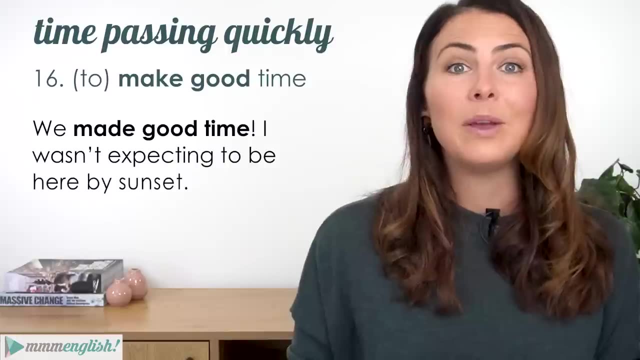 than you thought that you would, So you're making good time. Now I think we're about halfway there. We're making good time, Or you could say we made good time. I wasn't expecting to be here by sunset To make up for lost time. 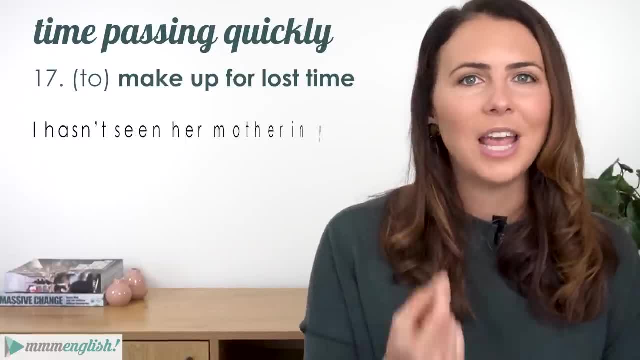 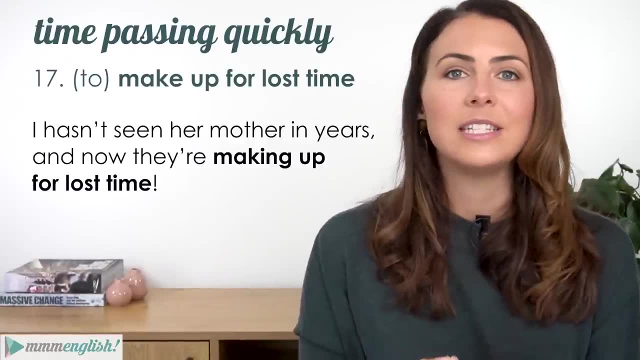 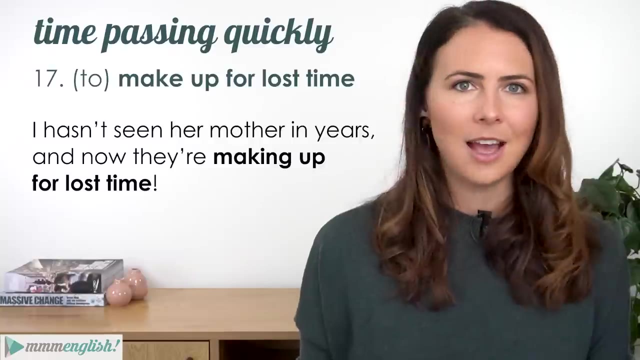 Now this expression is a really specific one. She hasn't seen her mother in years, and now they're making up for lost time. She missed out on seeing her mum for many, many years and now, finally, they're spending some time together, lots of time together, and they do it. 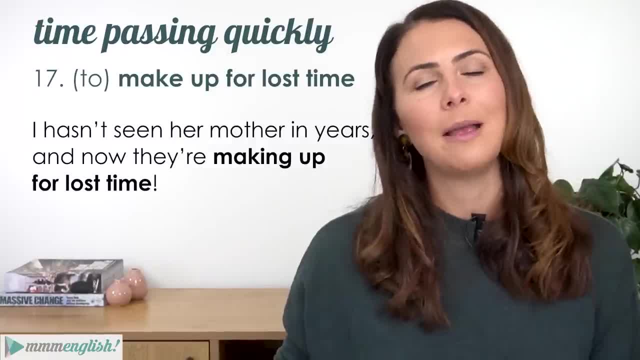 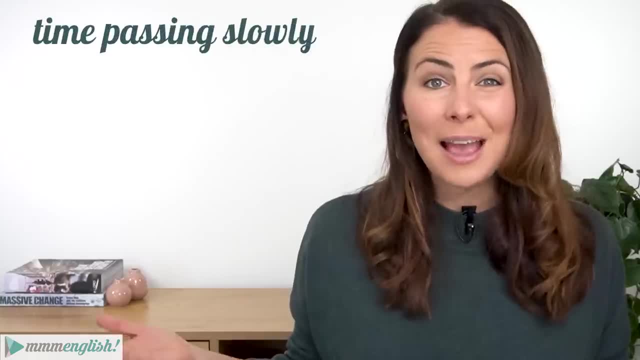 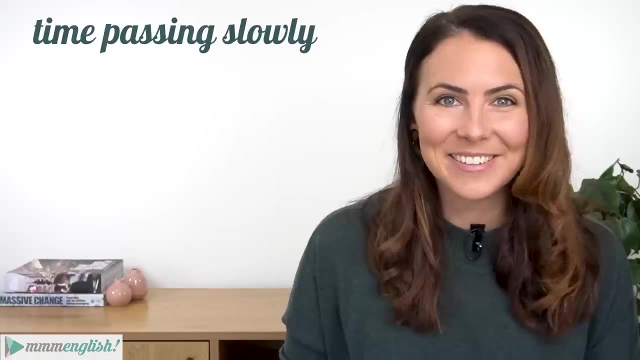 more often to make up for the time that they didn't have before. Really good one to know To make up for lost time. Now, time doesn't always pass quickly. Sometimes it passes so slowly, but hopefully that's not the case now. 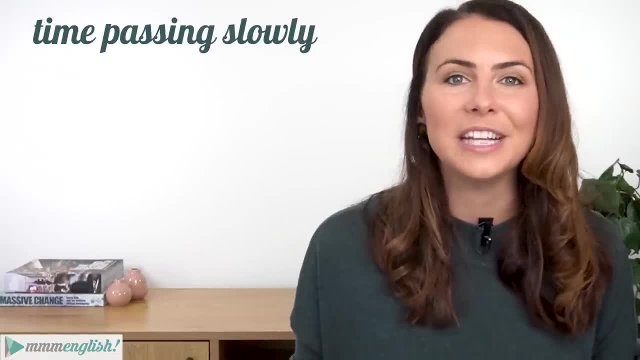 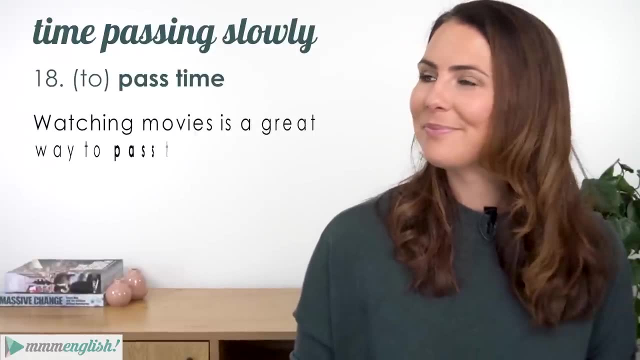 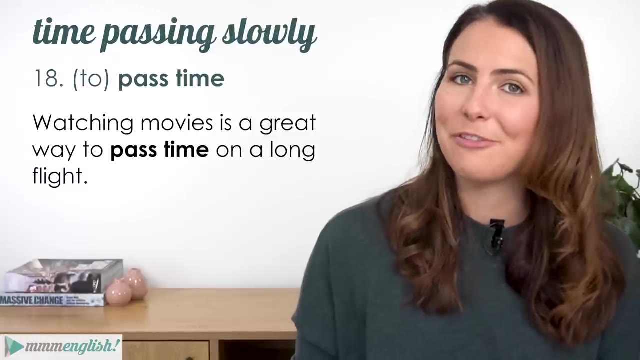 So usually if you want time to go faster, to feel faster, then you need to do something to keep yourself busy for a while, To pass time. Watching movies is a great way to pass time on a long flight. A more informal version of that same phrase is to kill time. 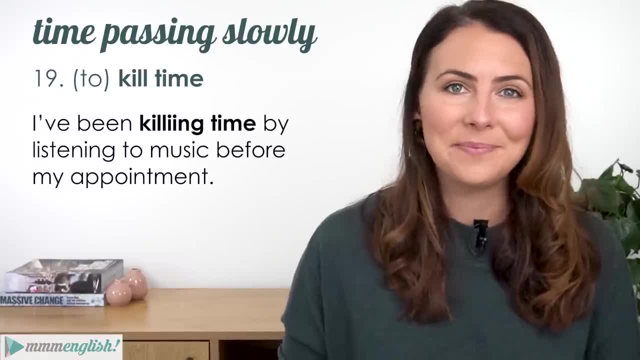 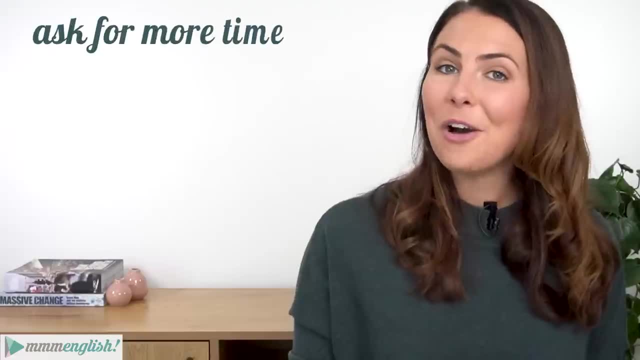 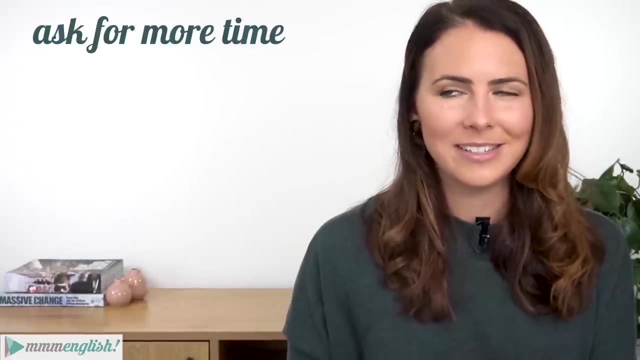 I've been killing time by listening to music before my appointment. Now it sounds kind of violent, doesn't it? But it's not. This is just an expression. Now, we often need to ask for more time, don't we? When things are happening too quickly or too many things are happening at once. 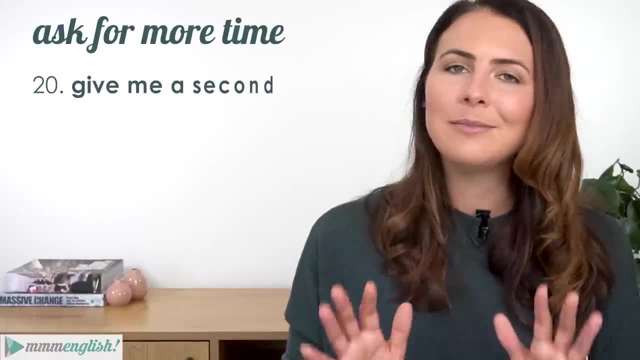 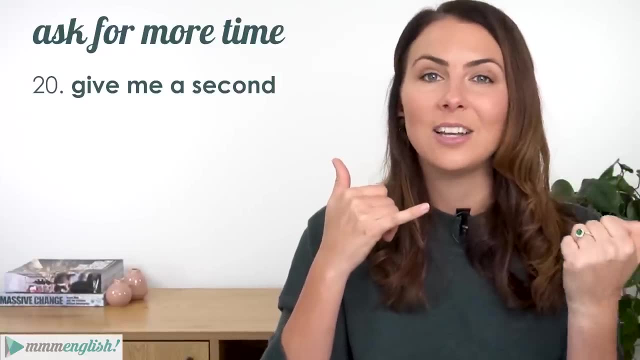 So often you need to ask someone politely to wait. So imagine I'm on the phone and I'm speaking with someone and at the same time you come up to me to ask a question and I might say to you: just give me a second, I'm on the phone. 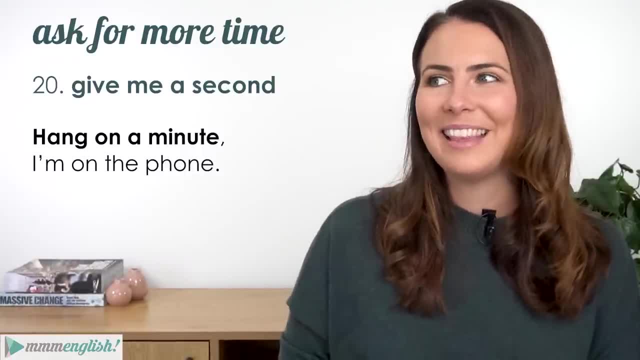 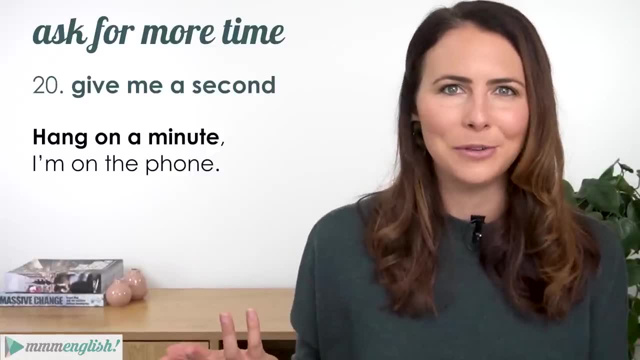 Or hang on a minute. I'm on the phone Now. we always use a second or a minute in these expressions like a second is all of the time that you need. It doesn't really matter, It's just a way of asking for more time, for extra time. 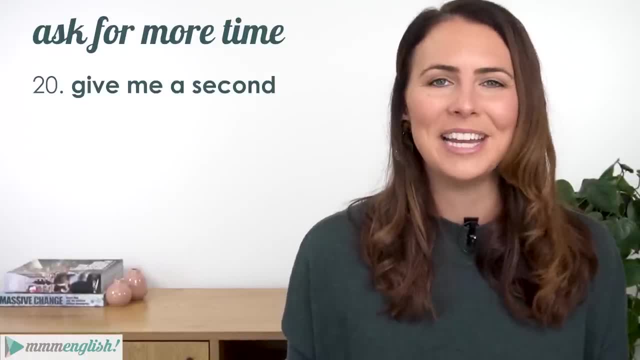 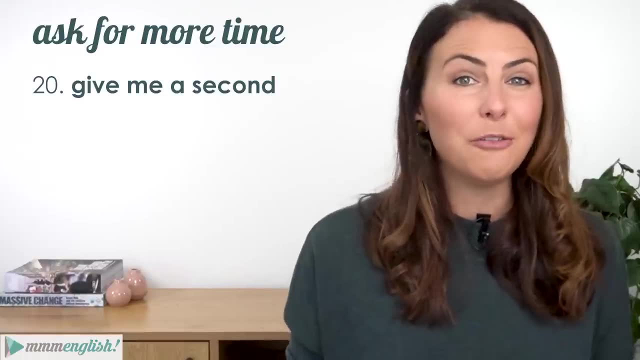 So, even if it sounds ridiculous, it doesn't matter. You might need more than a minute or more than a second, but it's okay. In fact, if you're speaking sort of informally with someone, the lazier version of that is to say: give me a second. 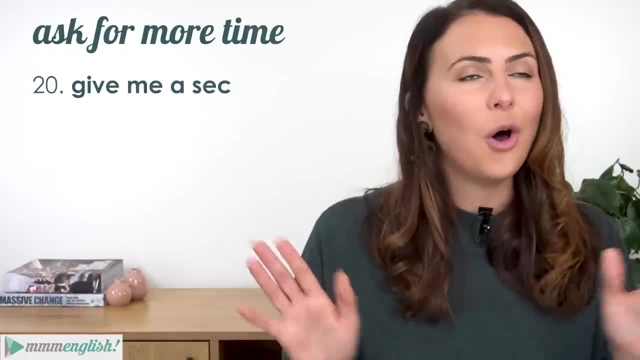 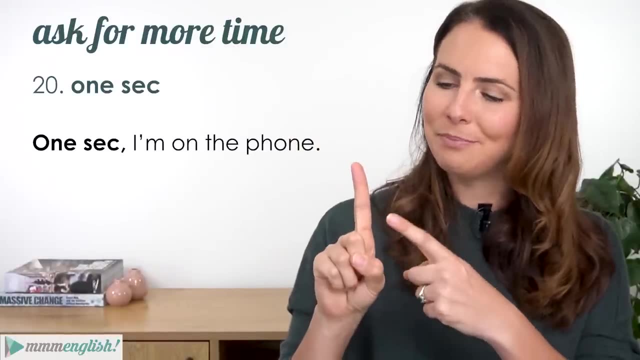 And if you want to be even lazier again, then you can shorten the whole expression to one sec. One sec I'm on the phone, And that's important body language. One sec I'm on the phone. Or you could say just a sec: I can't find my keys. 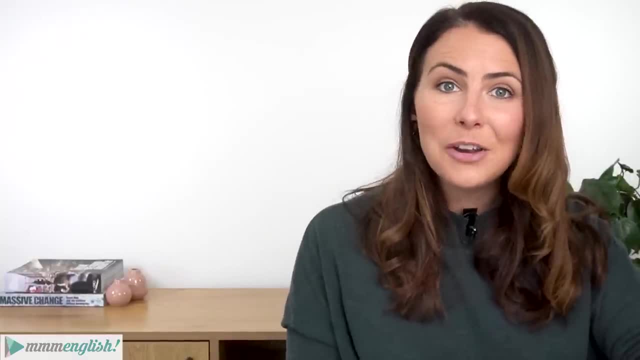 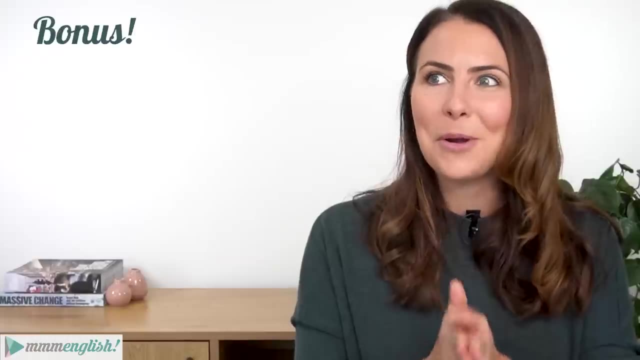 Are we making good time? Oh no, we're almost out of time. But for those of you who have stuck with me all the way through, I've got some really awesome bonus idioms and examples. I've got some really awesome bonus idioms and examples. 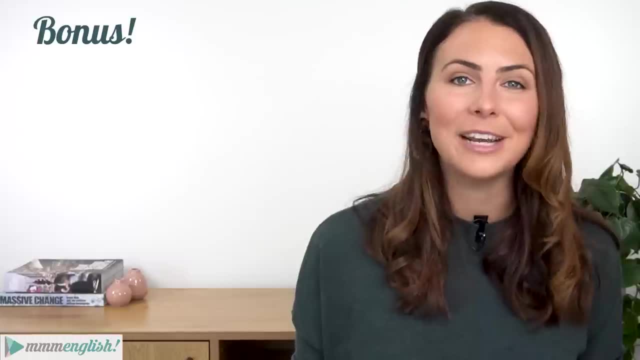 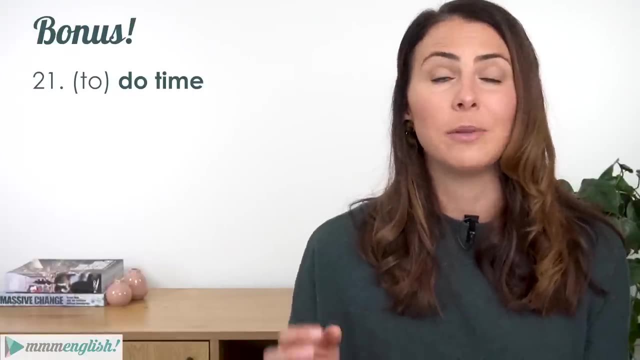 I've got some really awesome bonus idioms and expressions for you, ones that are really useful, really common expressions, Like this one: to do time. Now, this sounds really general, but it has a very specific meaning: To do time is to spend time in prison. 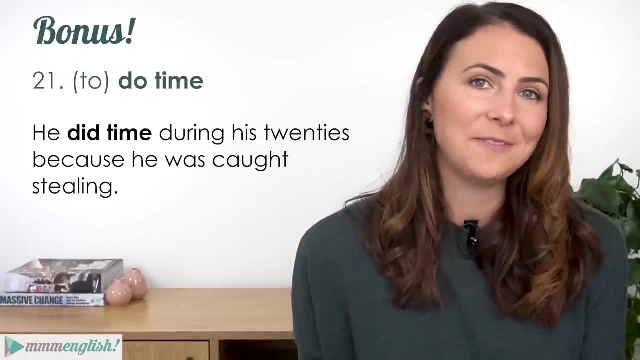 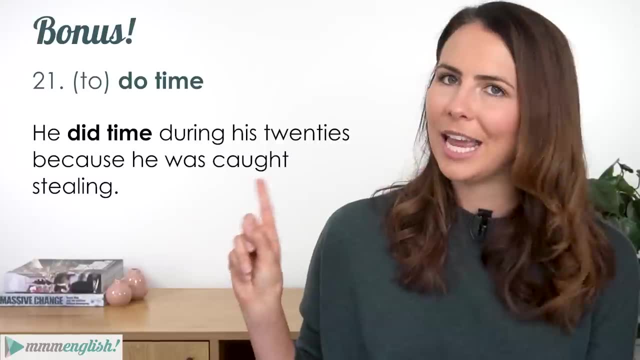 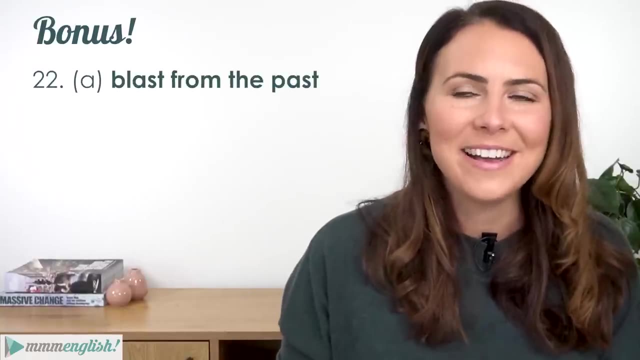 He did time during his twenties because he was caught stealing. Now that is definitely one verb that you don't want to mistake right, An important collocation, because it's only really used in that context to talk about someone in jail, A blast from the past. 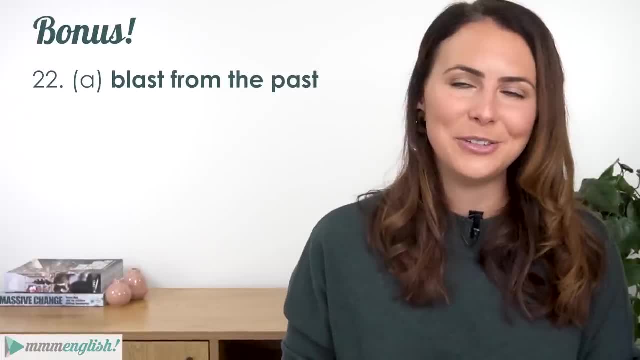 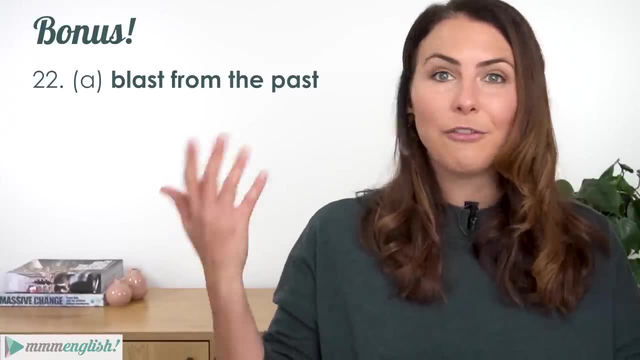 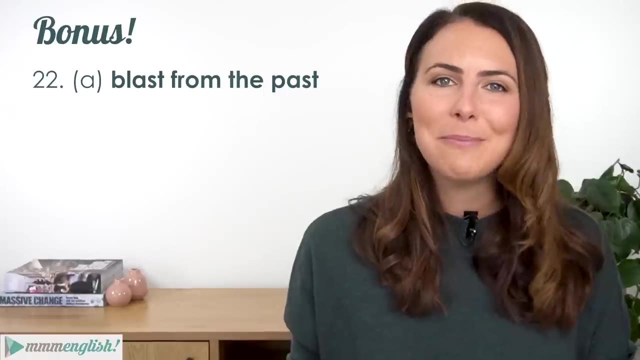 Now, this is a really fun expression that I love to use. A blast from the past is kind of what it sounds like. It's something or someone from your past who pops up and surprises you in the present moment. So it usually brings back fond memories, or positive memories. 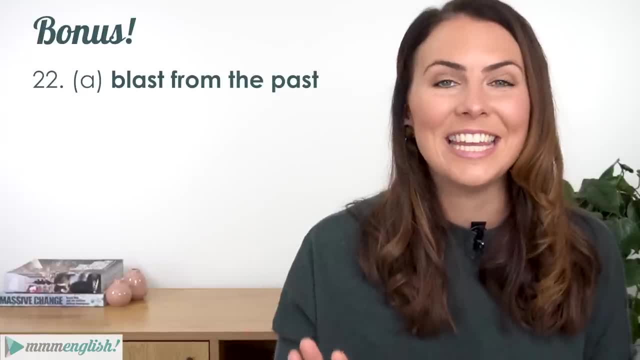 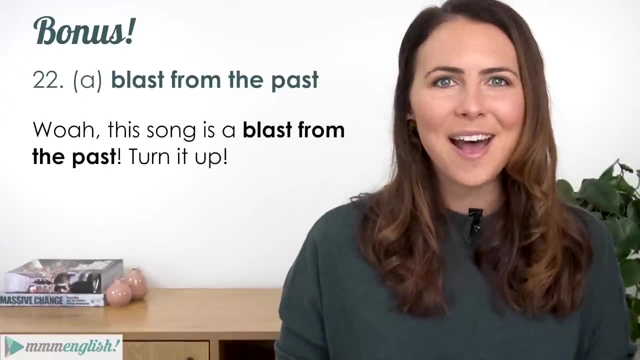 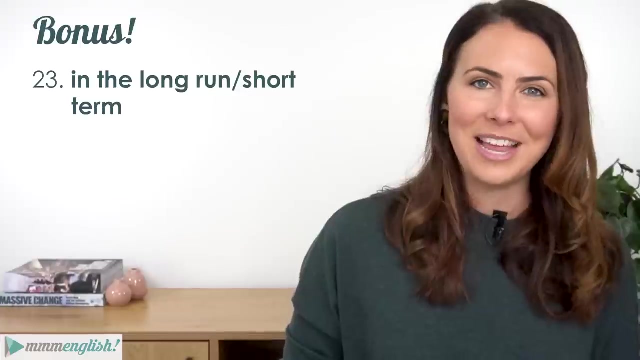 It's like if a favourite song that you haven't heard in years comes onto the radio, then you might say: Well, this song is a blast from the past, turn it up Now. these expressions are both useful and very common in the workplace. 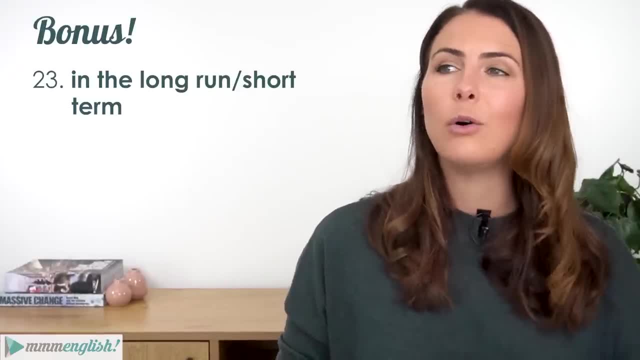 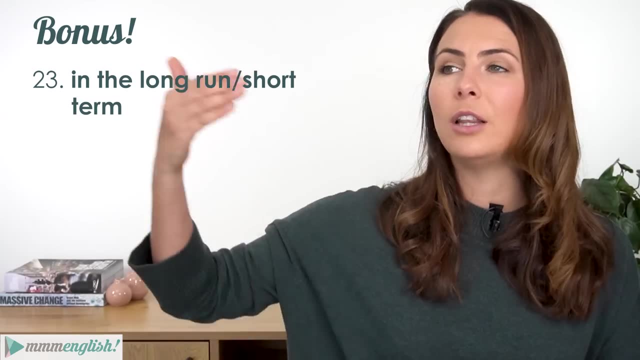 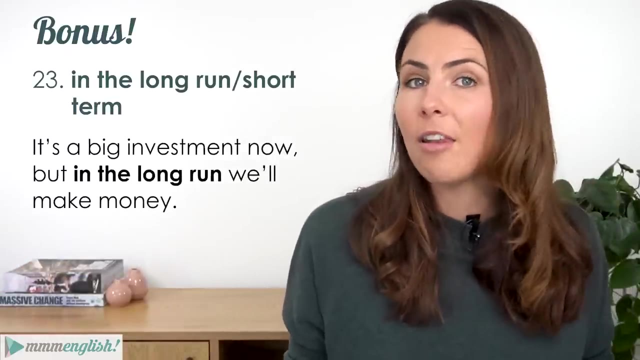 So when you're presenting or you're giving an opinion or you're trying to summarise something, these can be so helpful. In the long run means over a long period of time where eventually something will happen. It's a big investment now, but in the long run we'll make money. 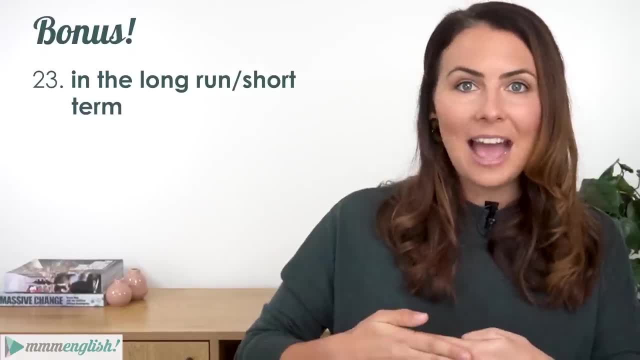 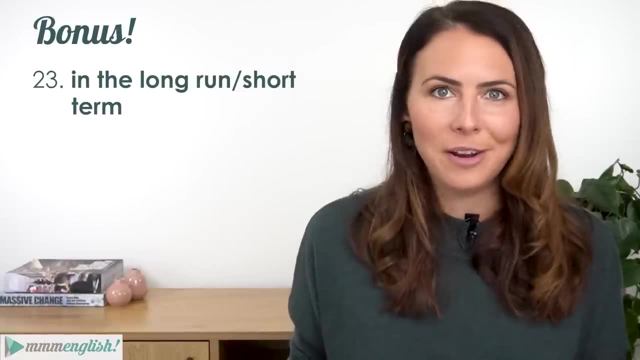 Now in the short term is the opposite: right From now until a point in the near future, So it's probably months, not years, which is the long run. This space is going to work in the short term, but we'll need a bigger place eventually. 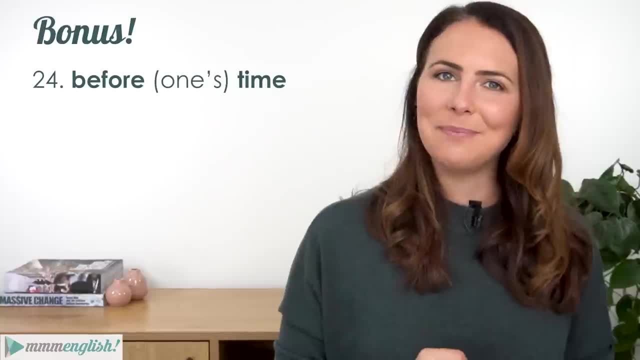 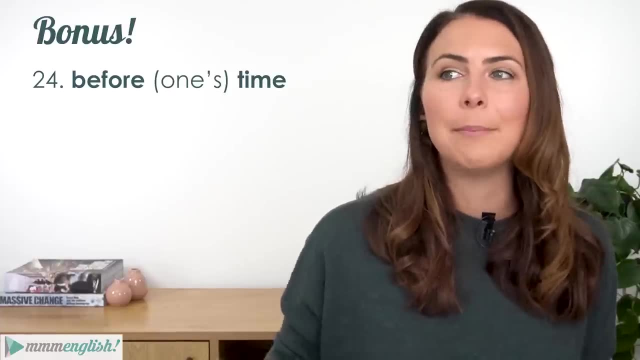 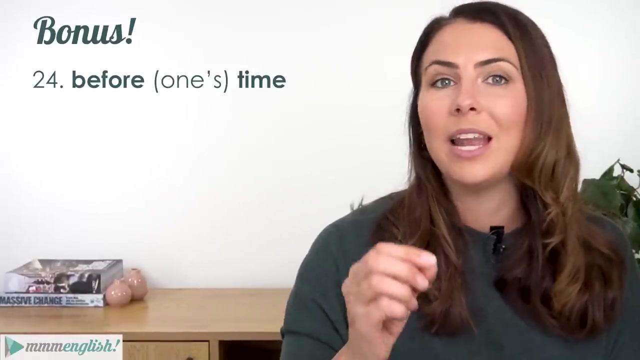 All right, here's the last one: Before your time- And this is an expression that kids really get tired of hearing, because before your time means something that happened before you were born or just before you were paying attention, And you could say this to someone as a reason why. 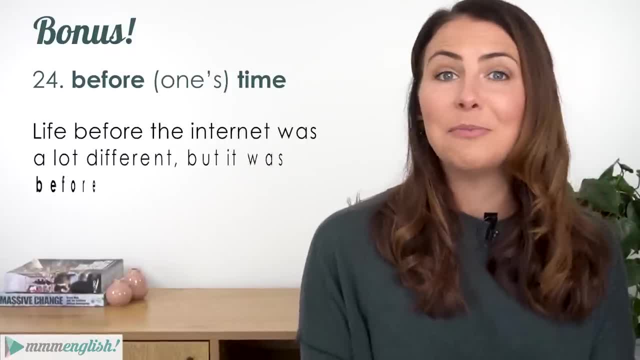 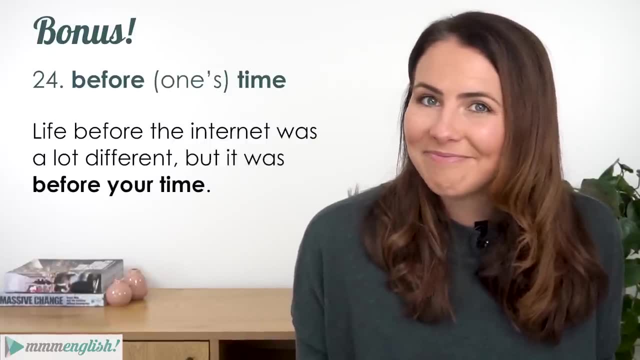 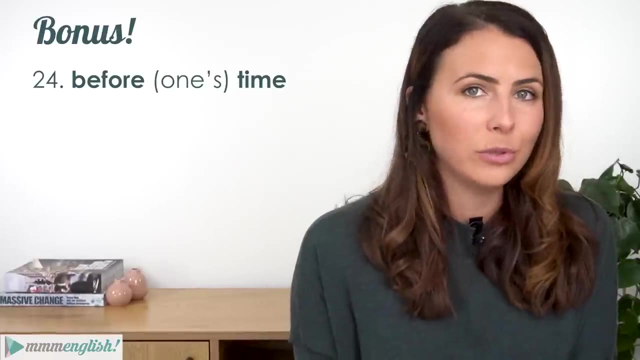 they don't understand something you know. Life before the internet was a lot different, but it was before your time so you wouldn't understand. Or you can say it about yourself as an excuse why you don't understand something or why you don't know something.